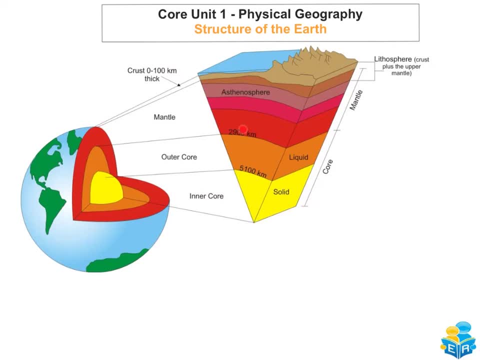 Mantle. Okay, the Mantle and the Crust, which we'll talk about now, But the Mantle itself surrounds the Core and it's the largest layer. About 80% of the Earth's volume is the Mantle. Okay, so it goes from here to here. Rocks are in a molten or semi-molten state Now. you can see the Crust on the surface. That means the Earth is excessively hot and there are a lot of rocks around the Crust. It's not a big amount of rock in the Crust. You can see that the Crust is very hot because of the ice, So the Crust is very hot And the Crust is. 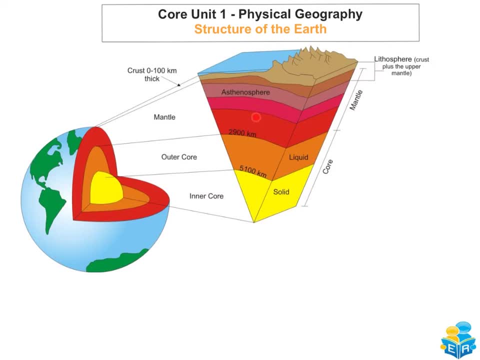 molten state part of the mantle is known as the asthenosphere. okay, which is up here, the asthenosphere is the top part of the mantle. okay, that's the asthenosphere. it's the top part of the mantle and the rocks in the asthenosphere which is just here are much weaker and almost. 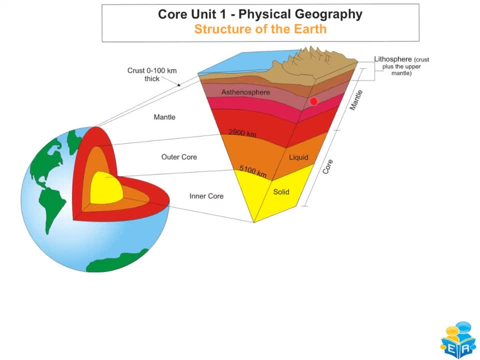 molten and they can easily change and are capable of like flowing, and so in the asthenosphere you have, like, the convection currents. this explains to us why the plates actually move. then up here we have the litmosphere. so the litmosphere makes up the very, very top part of the mantle and the 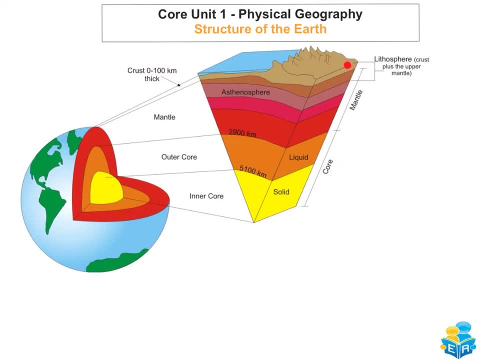 crust. okay, so it's the upper part of the mantle and the crust, and that is what is known as the litmosphere, but the top layer itself is just known as the crust. okay, and the crust is the earth's outer skin. 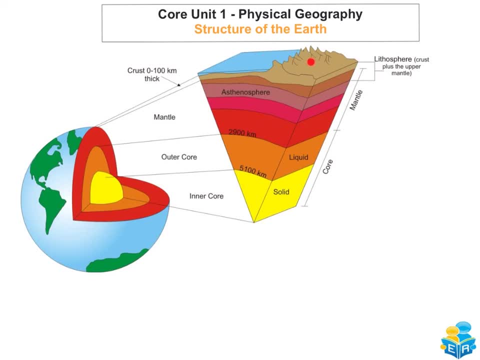 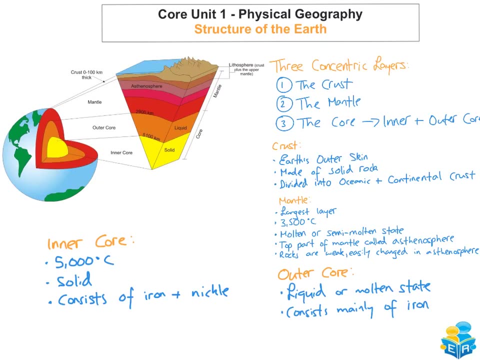 it's made up of solid rock, it's what we actually, it's what we live on, and it's divided into oceanic crust and continental crust. Okay, so I've wrote out the few different points that I made about each one. first of all, the inner core: up to 5000 degrees solid in temperature, it's solid. 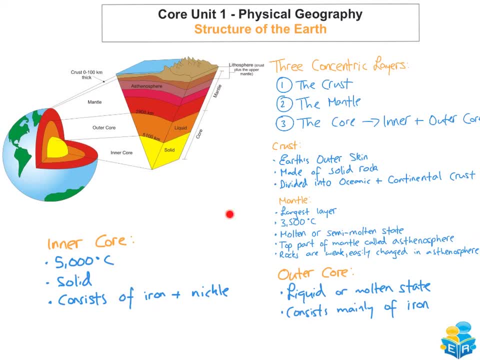 because of the pressure and it consists mainly of iron and nickel. the outer core, which is the liquid or semi-molten state, that's because there's less pressure and consists mainly of iron. in the mantle it's the largest layer. it makes up about 8% of the earth's volume. 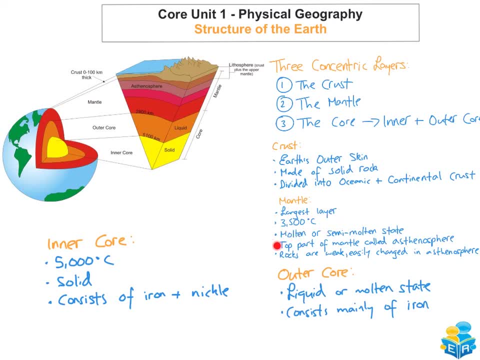 temperatures here reach up to three and a half thousand degrees celsius. the rock is molten in a semi-molten state. the top part of it is known as the asthenosphere and this is a very weak part and it's easily changed. rocks are easily changed in an asthenosphere and almost like a flow in.